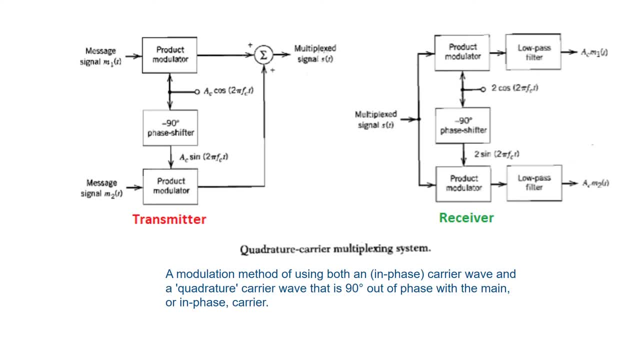 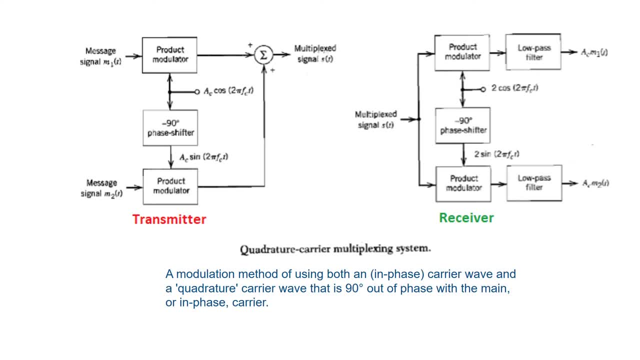 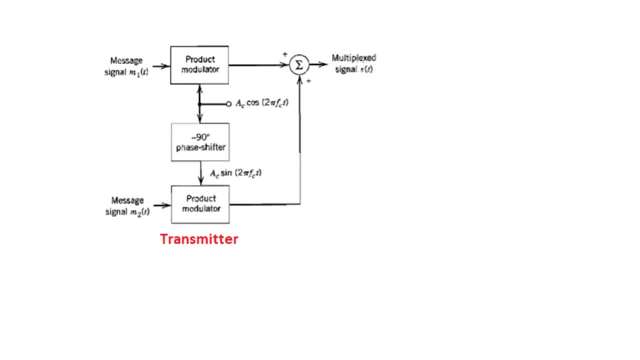 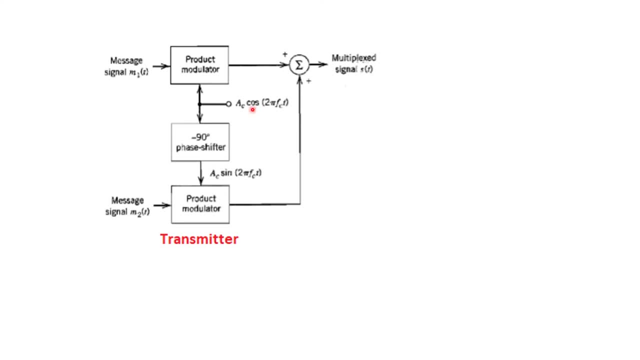 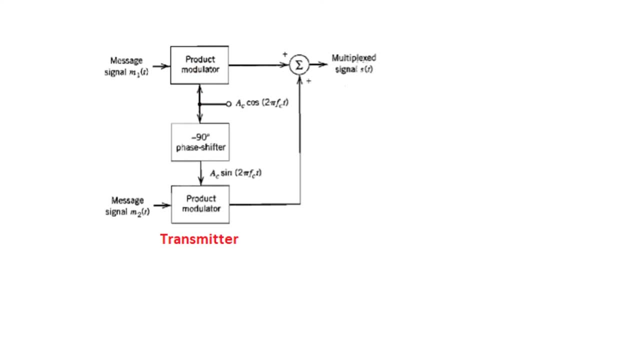 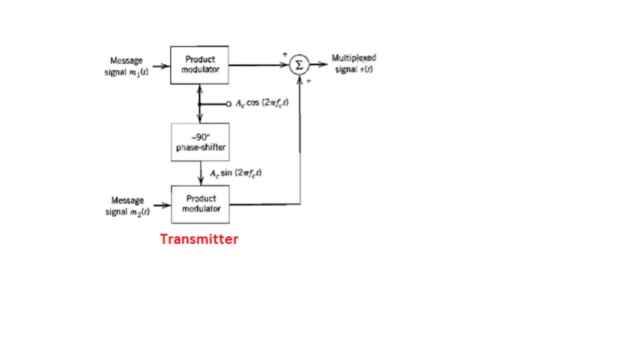 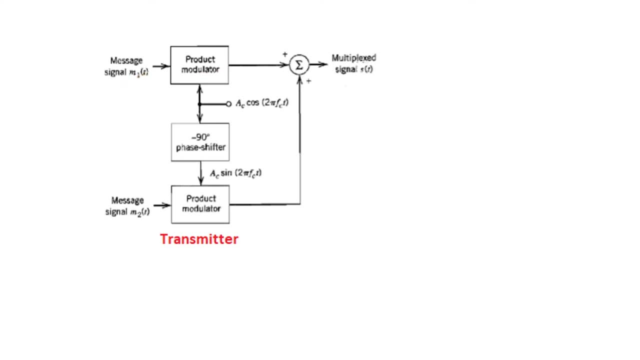 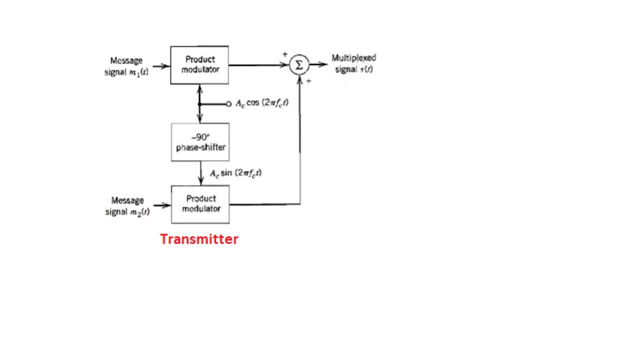 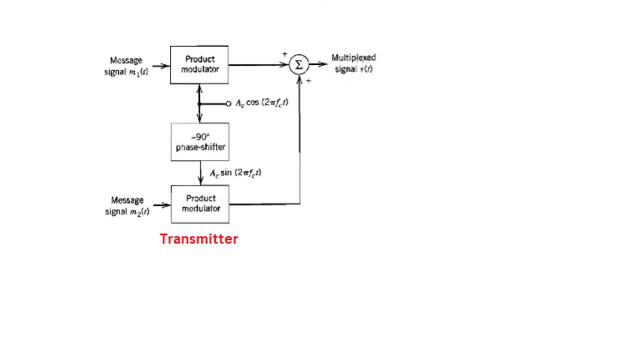 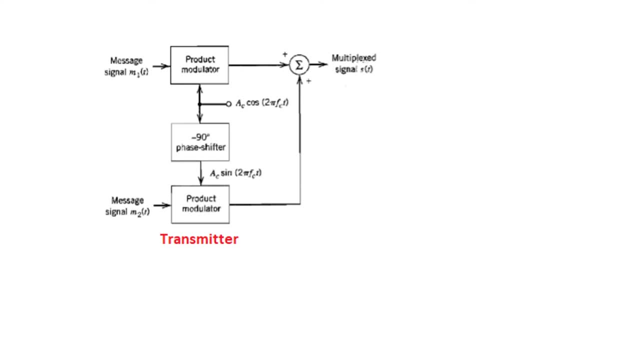 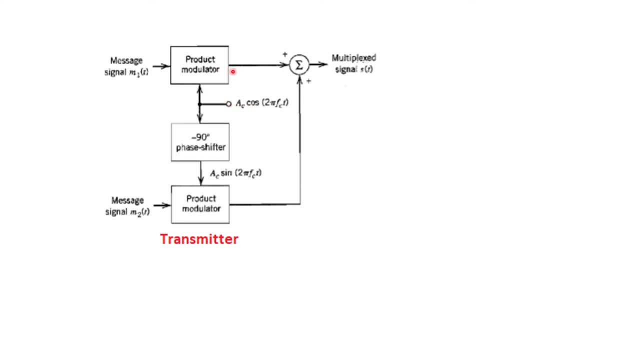 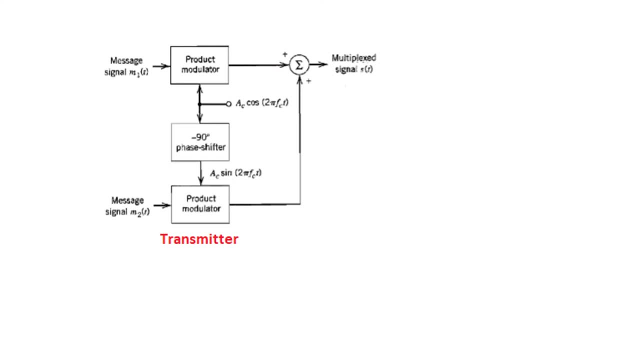 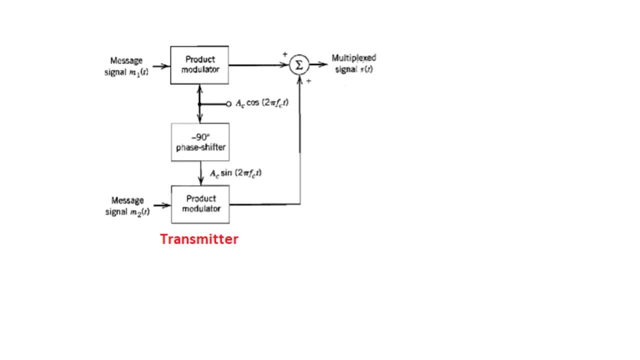 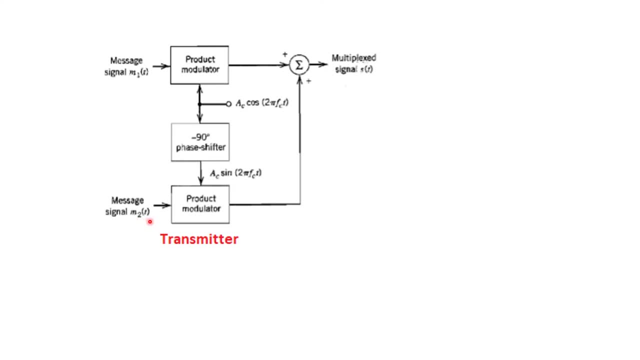 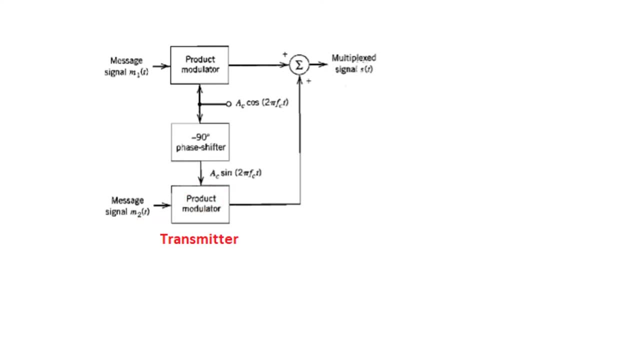 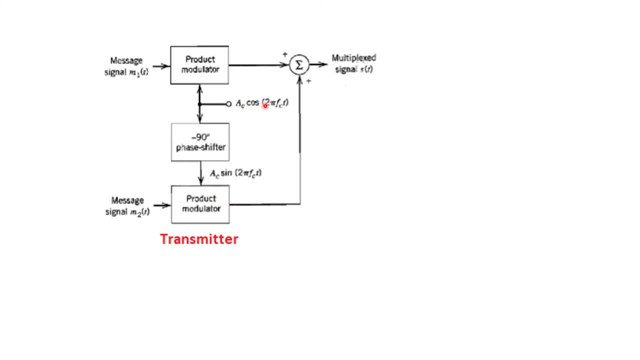 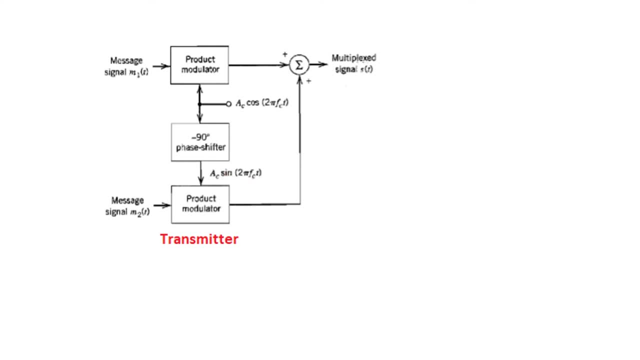 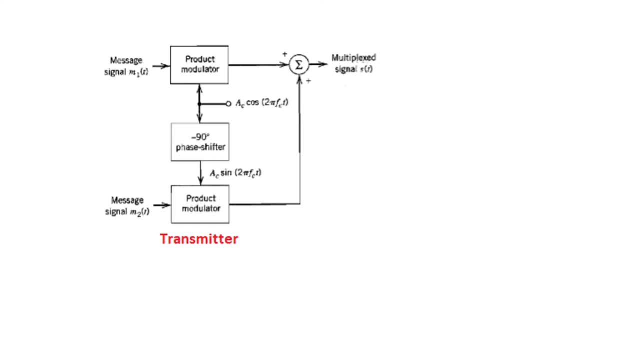 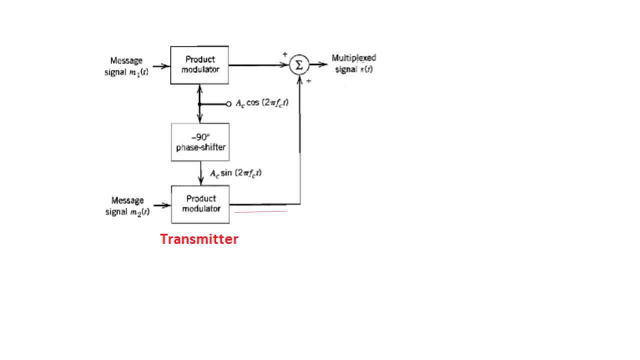 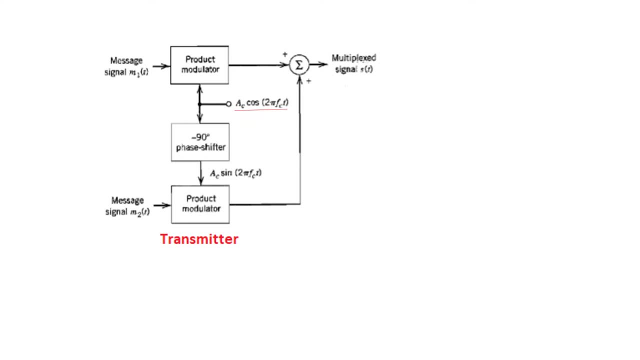 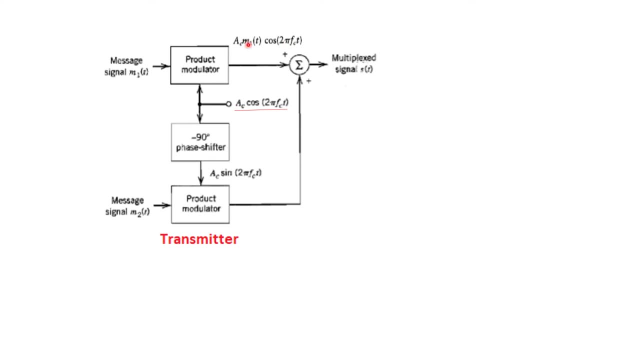 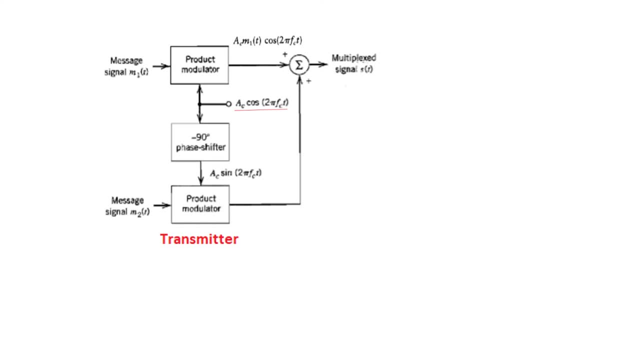 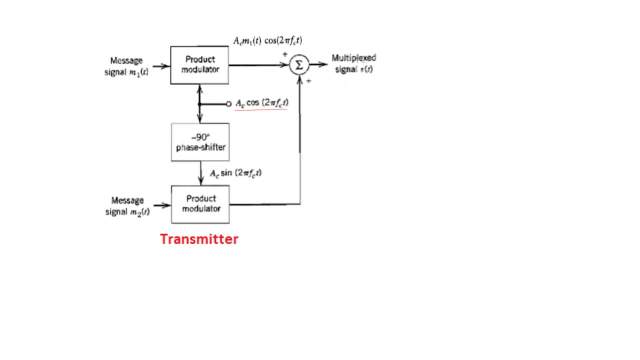 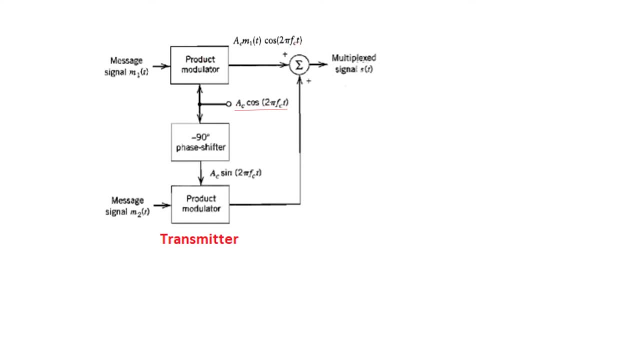 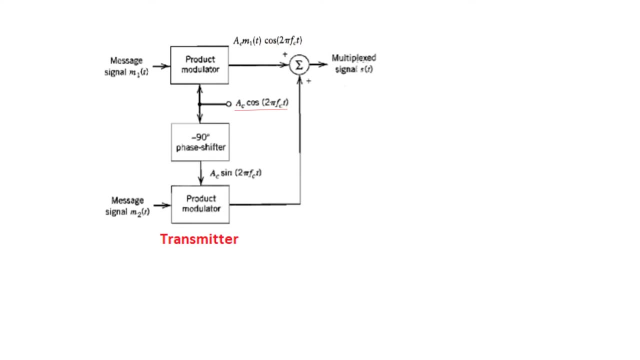 This is our carrier wave in the transmitter and also in the receiver. This is our carrier wave in the transmitter and also in the receiver. So this is the in-phase component, and the quadrature component is the multiplication of these two, and so our output will be the summation of the two. 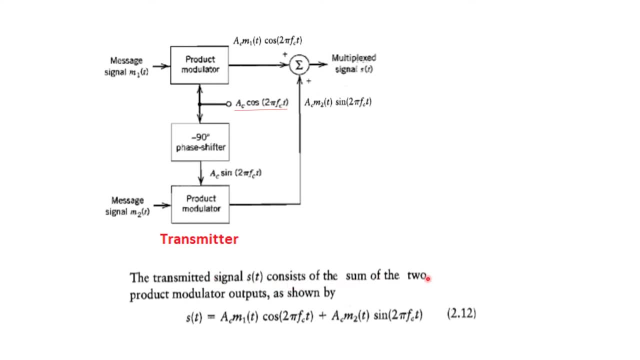 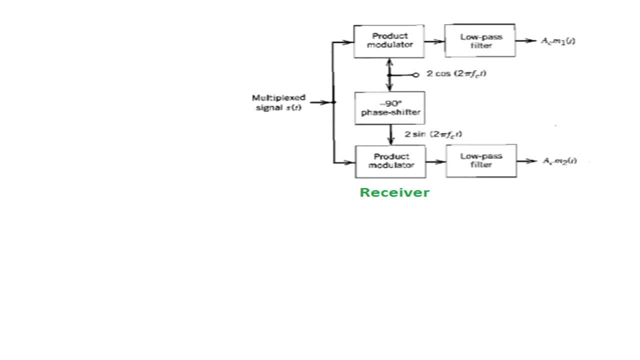 So the transmitted signal S t consists of the sum of the two product modulators, so sum of the top one plus bottom one, or in-phase and quadrature component. Now at the receiver end we are receiving the signal which we are transmitted. so this was. 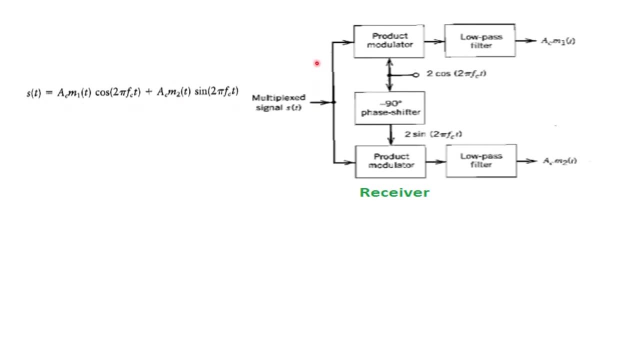 the transmitted signal. So this signal is now going to the both top modulator, or in-phase modulator, and the quadrature modulator or the bottom modulator, And exactly similar Arrangement is here. we have a carrier signal and it is going directly to the product modulator. 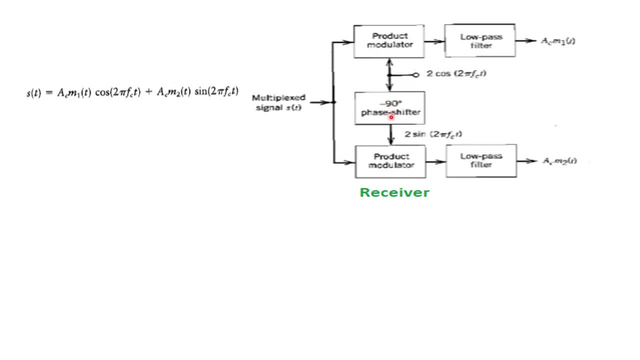 and after 90 degree phase shift it is coming to the quadrature product modulator or the lower product modulator And then they are passing through two low-pass filters to recover the original signal that we had sent. So it went directly to the minus one mid-pass filter and the fare that we have received. 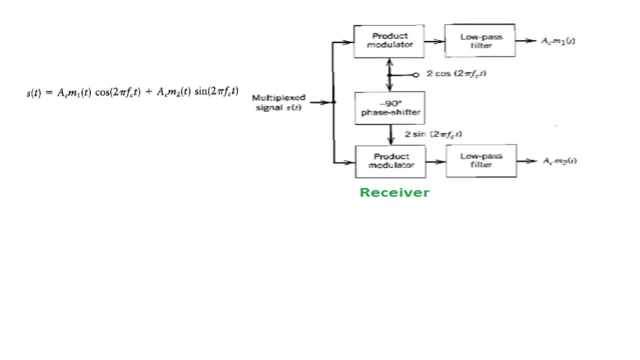 in-phase modulator is directly to the Qi-fan filter. So we are in-phase modulator off the bottom of the m1-t at the top and m2t at the bottom. Let us see some mathematical expression. So this signal going. we are just considering the top path and I hope you can do the same. 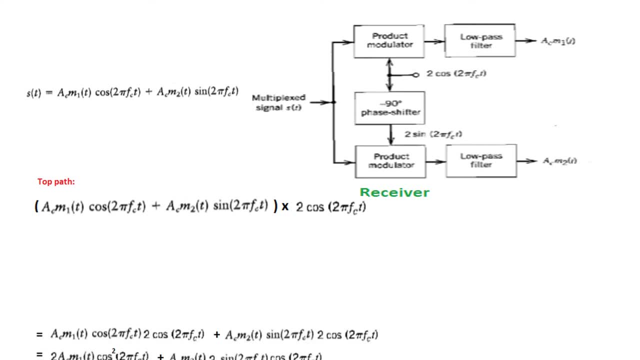 calculation for the bottom path. So the signal is going to the Billy. when to the product modulator. multiply it by the carrier, which is 2 cos, pi, f, c, t, and if you just multiply these terms you will get two separate terms and this cos, cos will. 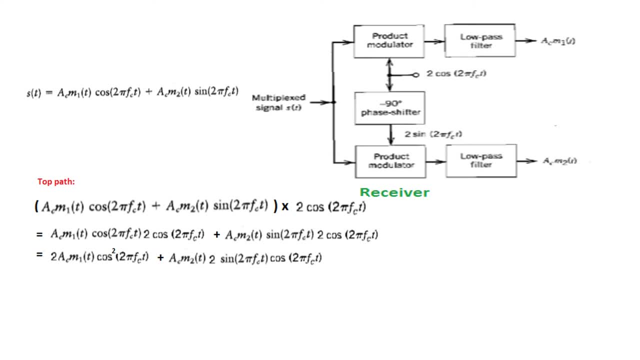 become cos square and here it will be sin and cos, so we can use the trigonometric formula. we will use this cos square alpha, this formula here, and two cos a, sin b or sin a- cos b formula for the second one. okay, so the first formula will result in the first part of this and 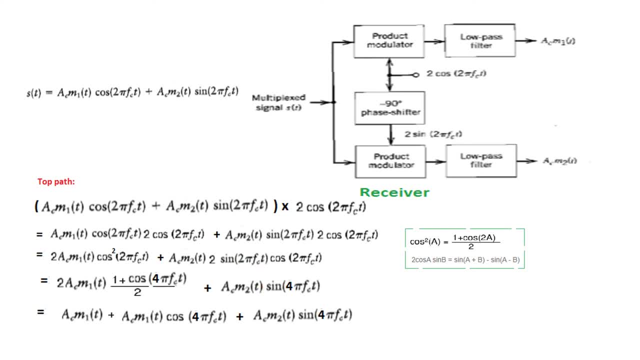 this will give to the second part and if we open this, this is the final shape that we are getting. now, if you look carefully, the frequency here is four fc three, four times the original carrier frequency, same here. So these are higher frequencies. Now, this is only the 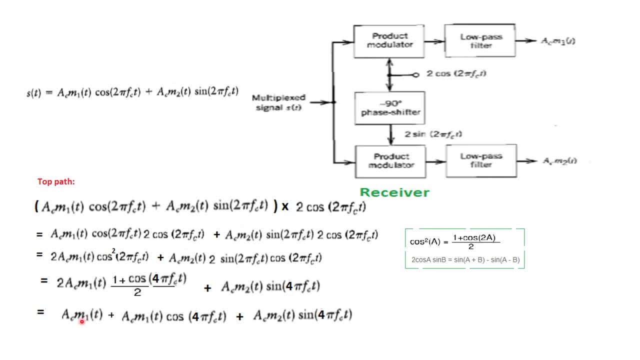 information bearing signal, which we say is audio, tone or something similar to that which is a low frequency component. So if this passes through the low pass filter, then what will happen is that the high frequency components will get eliminated, So these two get eliminated. So 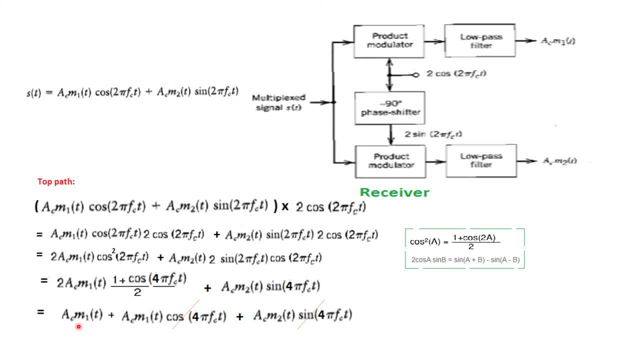 only the tone signal or the baseband signal will come out of the low pass filter. So this way we have been able to recover the first signal and exactly similar method of calculation. if you follow, you will be able to find that the second signal is also recovered. 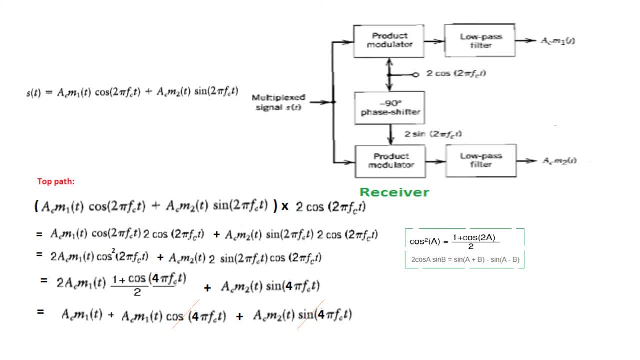 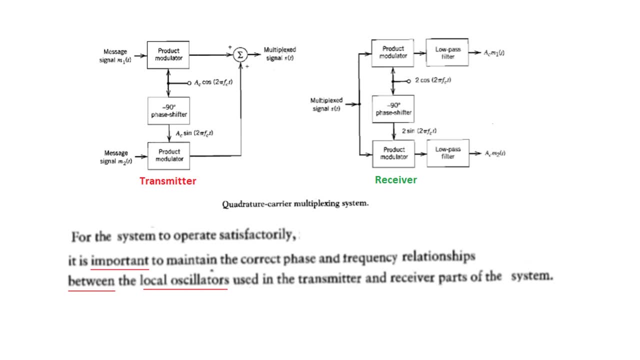 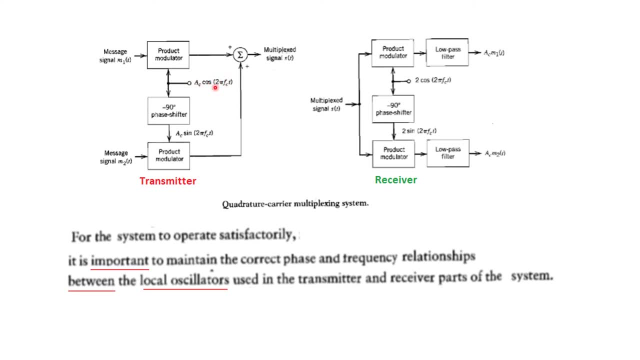 This is good. This is good. Now, if you remember that at mid frequency the carrier is generated at the transmitter, which may be very far away. So inside there are very similar frequencies And this carrier is generated at the receiver, So there could be more than one receiver. so many. 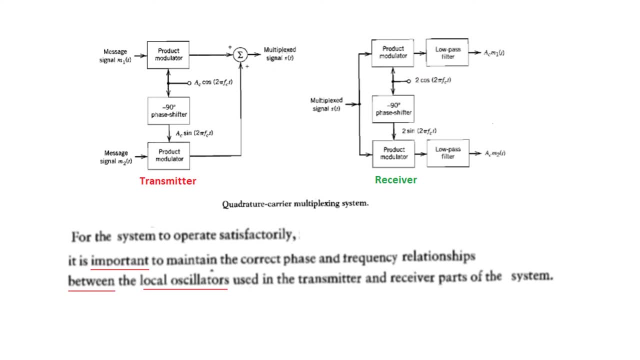 receivers. Now, important point is that these has to be similar, Same frequency and same phase, which is, of course, very, very difficult to generate or maintain because of the separation and Coastalever. I didn't break this. I kept hearing the same sound Instead of the other. 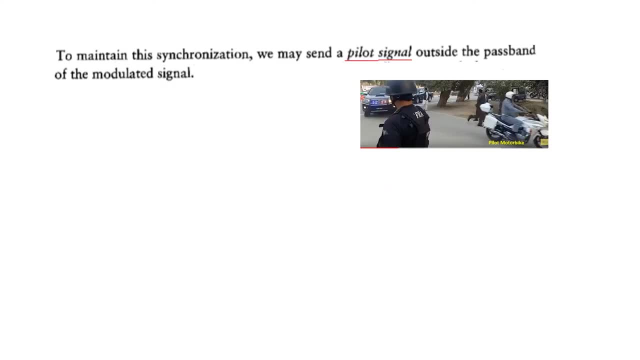 envelope, get away from Bronco and Messing. this could be different, even if you observe these the two. So what technique is followed is that we send a pilot signal, and pilot signal is, if you recall, VIP movements. it is led by a motorcycle rider who is called the pilot. 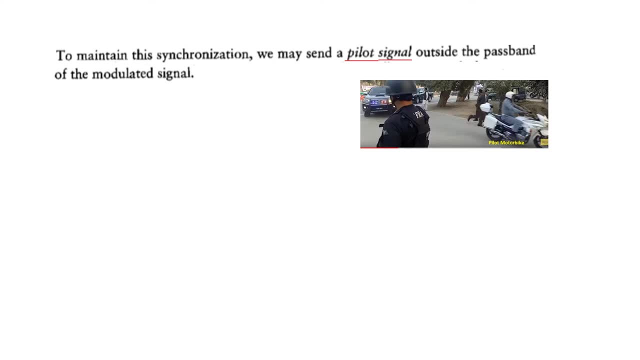 motorbike. So this kind of a synchronization or giving an idea that the VIP is coming. So same similar things we do here. In this method, a pilot signal typically consists of a lower power sinusoidal tone of a very low frequency, whose frequency and phase are: 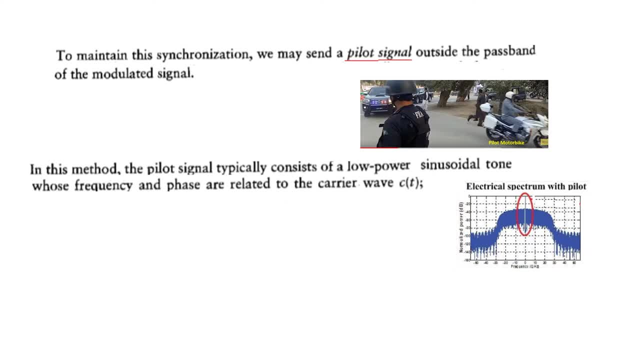 related to the carrier wave. So in the transmitter carrier wave is related with this tone signal from the transmitter which are transmitted and received at the receiver. So I could not find a very good Diagram but this here is showing that this is the pilot signal and went the carrier is. 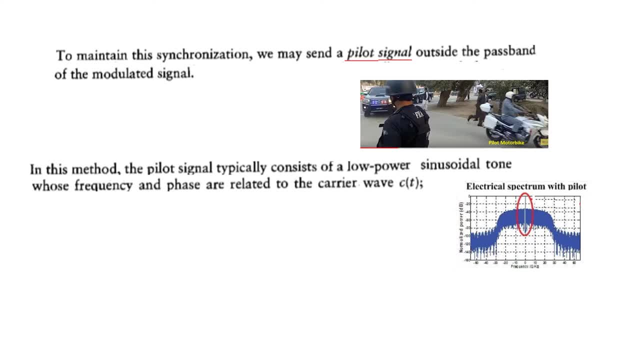 transmitted anyway. So when the pilot is received at the receiver, this pilot signal is extracted by means of a suitably tuned circuit- So there is separate tuned circuit for this- and then it is sent to the coherent detector Which then controls the frequency of the receiver local oscillator to match with that of the transmitter. 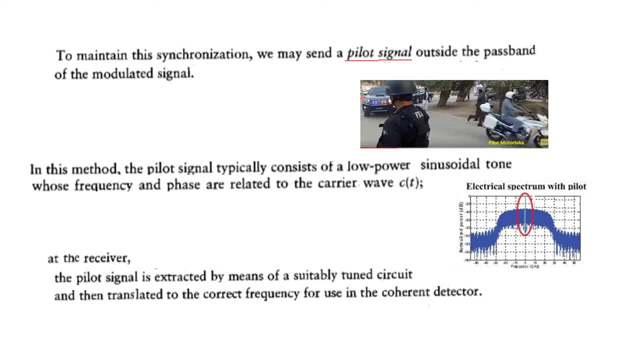 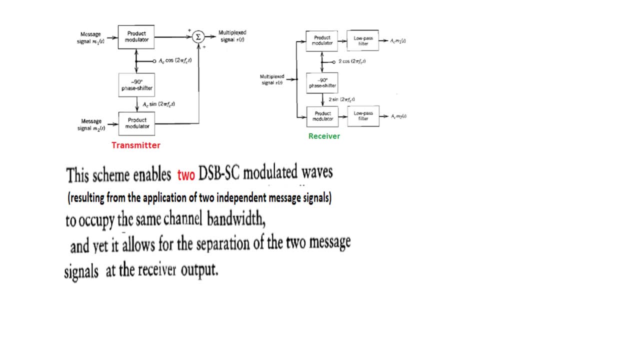 local oscillator. And now I comment. this scheme enables two DSBSC modulated waves. So these were the two DSB signals resulting from the application of two independent message signals. So two independent message signals, DSB, modulated here to occupy the same channel bandwidth. 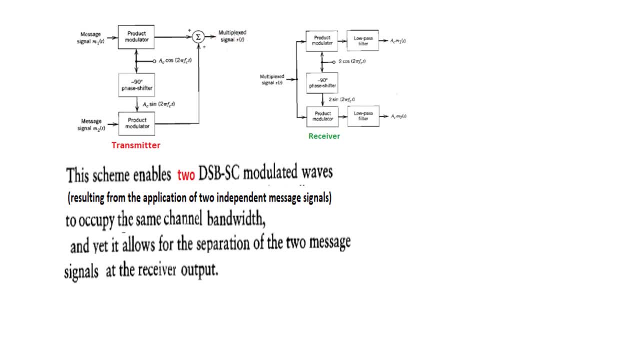 So they are going through the same channel, same path, and yet it allows the separation of the two message signals at the receiver. So although they are passing through the same path at the receiver end We have been able to detect them or separate them without much difficulty. So we can just to have an 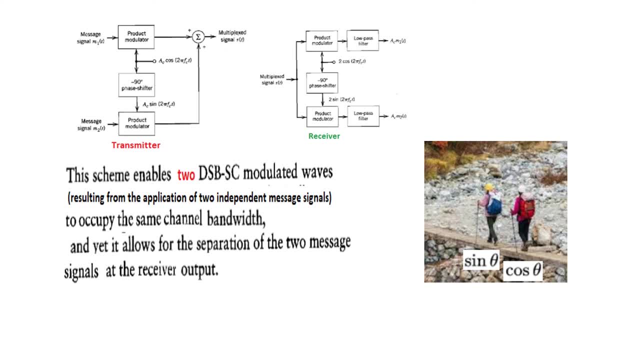 idea. we can say that if there is a narrow path, two people sine theta and cos theta. they are traveling and they can be easily separated, So they are using the same channel, same path. instead of a wider road, they are using the narrow path And that is why this method of quadrature modulator is called the bandwidth conservative. 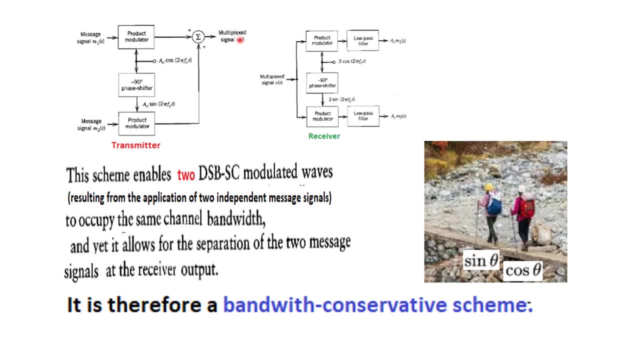 scheme. So what we have done, that we have used the only one bandwidth, one path, one channel, to send two signals. So they are conserving or saving the bandwidth. I hope this gives you some idea about the quadrature scheme. So thank you very much. Thank you.